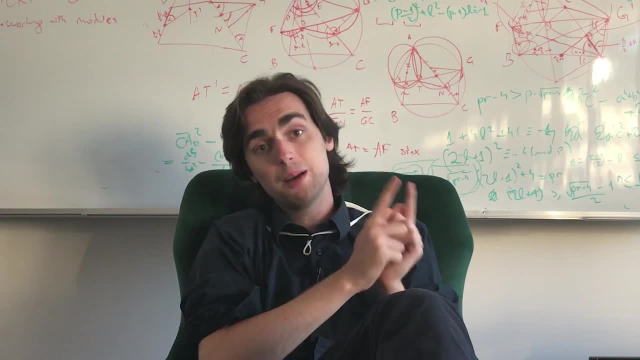 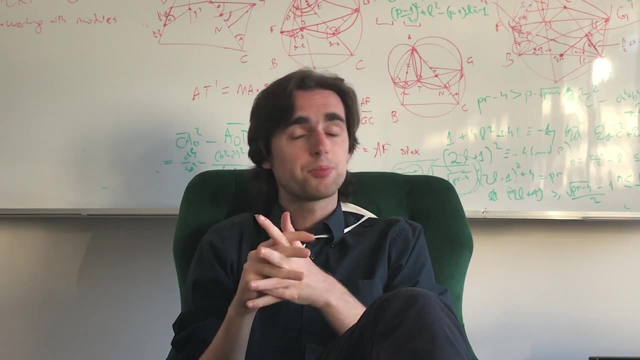 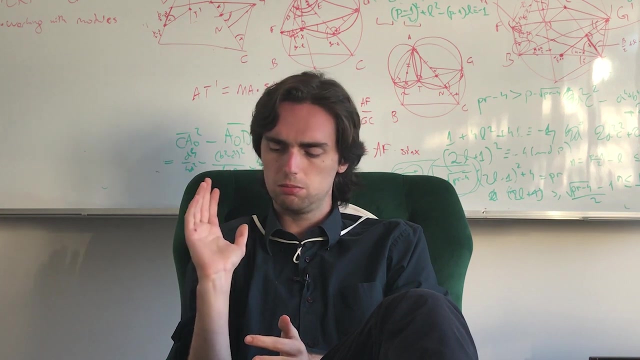 the exam. at the end of the day, what you're doing is solving problems. However, that being said, you can solve problems if you don't have the basic tools. So what is a good book that you can look at? So the first thing to say is: you just need a book that has a couple of things, Teaches you. 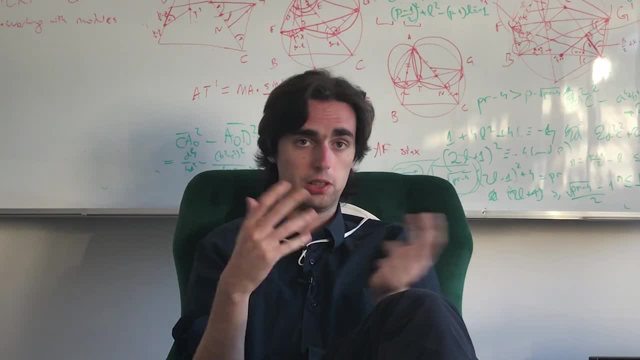 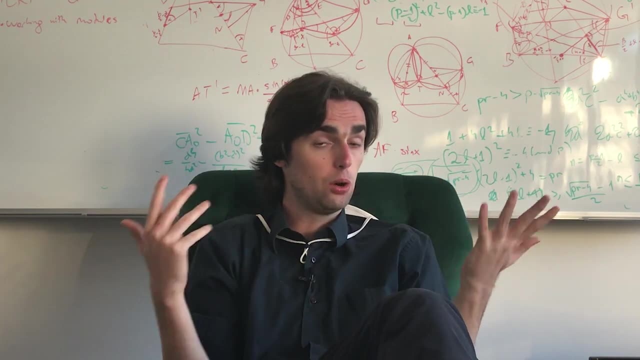 about congruence, similarity, angle chasing Tells you how to calculate angles, parallel lines. It teaches you about conciclic points, What is a circle and what are the things we know about circles With that, and these are the basics with which you can. 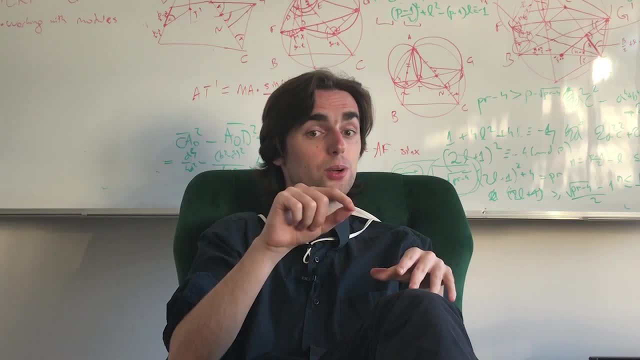 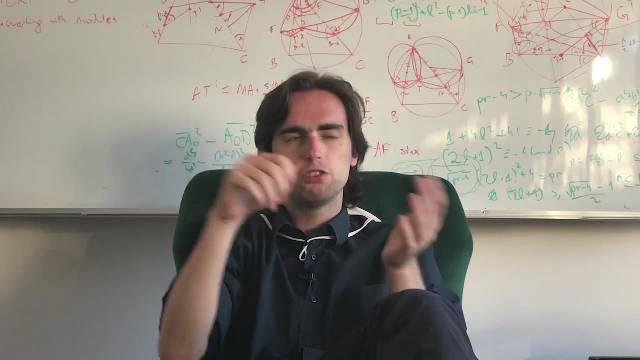 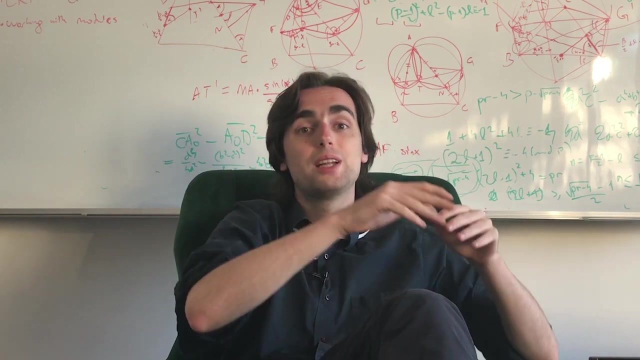 solve problems. So let's get started. A lot of problems, and it shows you a couple of places where it adds a point to prove something And after that sort of beginner layer, then it maybe teaches you a bit about trigonometry, which is an advanced concept which you shouldn't really try to learn unless you've already. 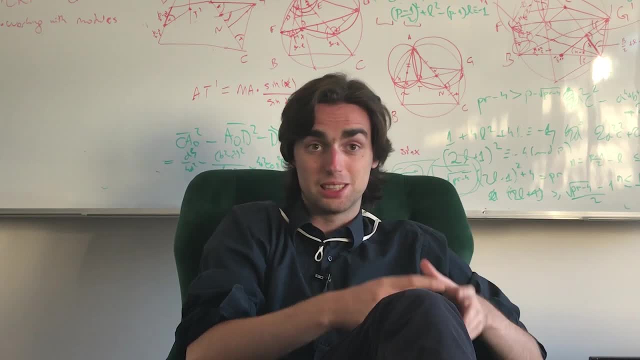 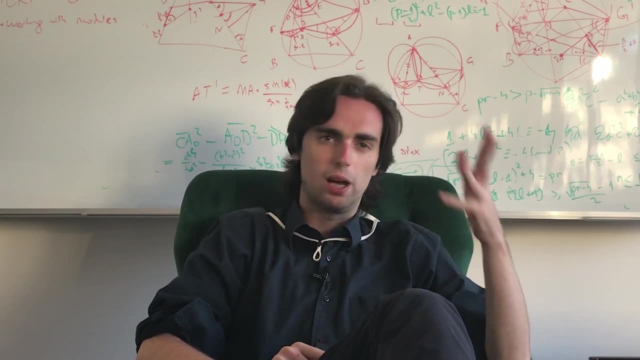 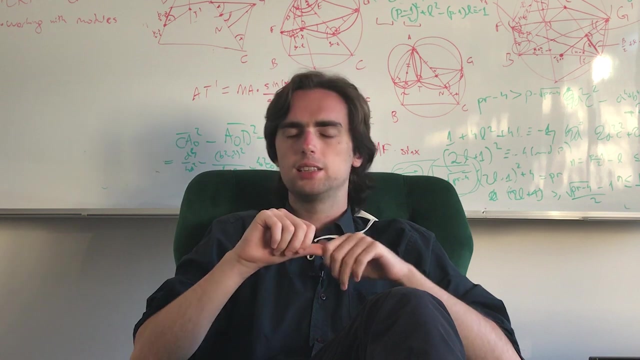 gotten very good at these other more basic concepts like similarity and congruence. So there's trigonometry, There is power of point, There's the radical axis theorem And with that homothetic as well, and Cheva's and Menelaus theorem. Now a good, maybe good book. 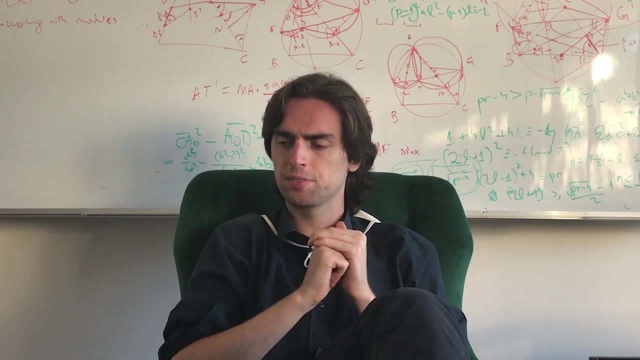 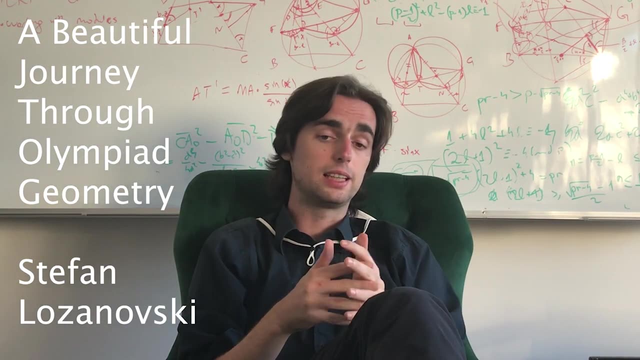 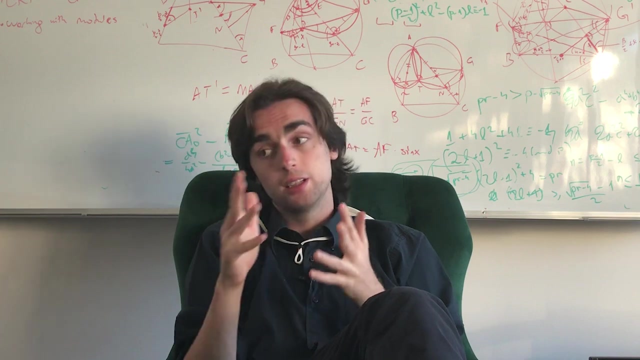 for this, which is, as of recording this video free, is A Beautiful Journey in Geometry by Stefan Lozanowski, And what that book gives you is it gives you all the really necessary theory that you will ever really, I believe, need for geometry. Now, that being said, there are other good books. 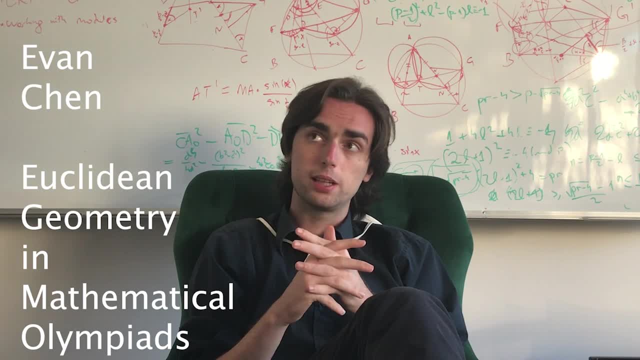 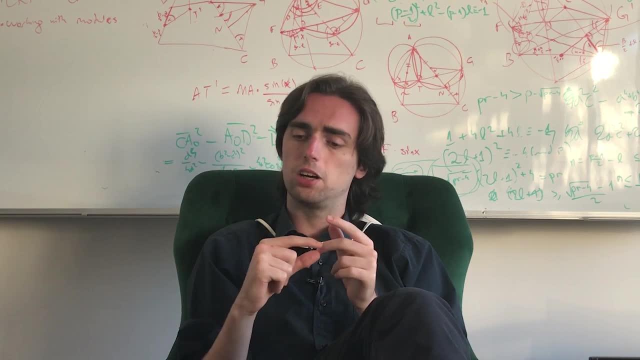 like Evan Chen's Element Euclidean Geometry for Math Olympiads or something like that, But that's a book you would need to pay. Other than that, there's Yufei Zhao's handouts are amazing. He has a handout on. 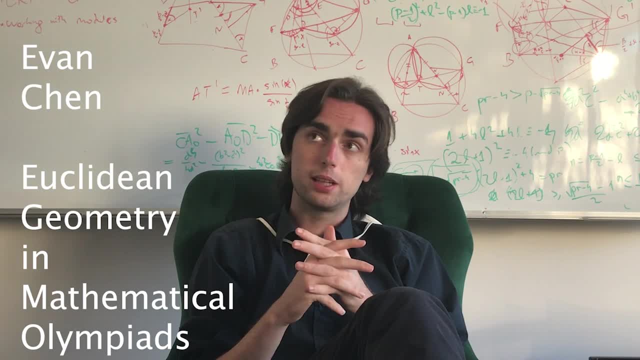 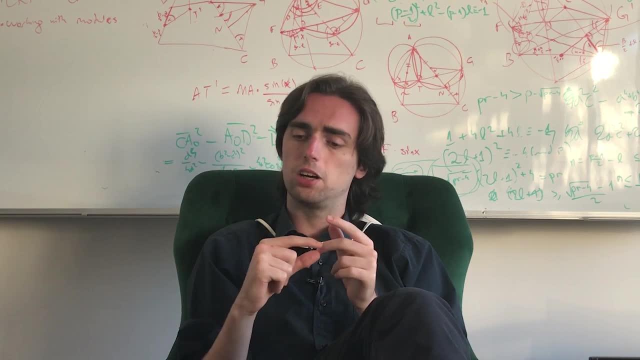 like Evan Chen's Element Euclidean Geometry for Math Olympiads or something like that, But that's a book you would need to pay. Other than that, there's Yufei Zhao's handouts are amazing. He has a handout on. 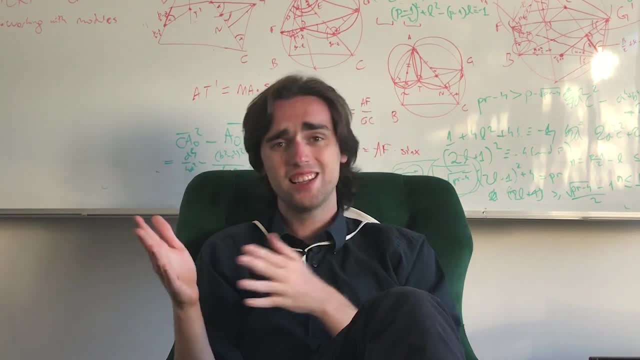 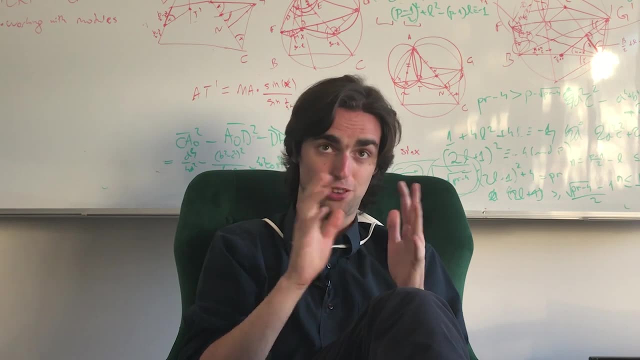 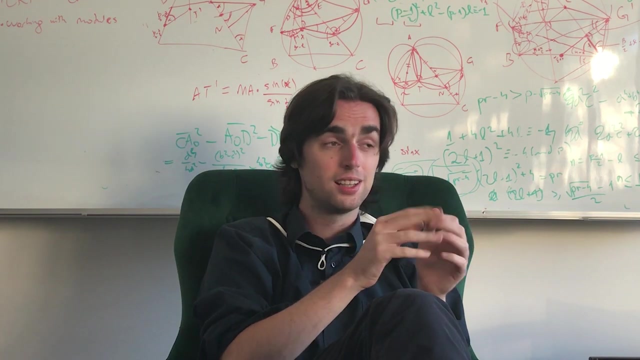 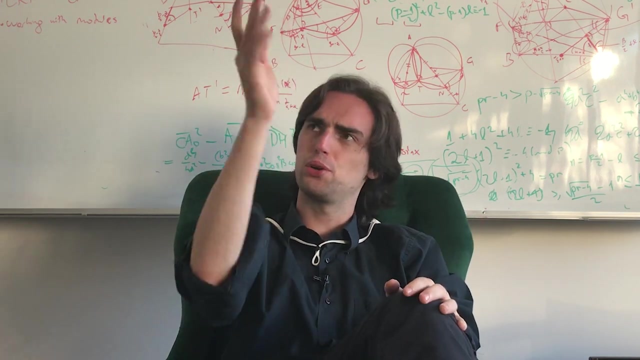 geometric lemmas, which is pure gold, And other than that, you need to solve problems, as with everything, And a good competition for geometry Olympiads- actually for geometry types of problems- are the Iranian Geometry Olympiad. This actually exists. It's a competition that only has geometry problems and you can stratosol problems from there in three or 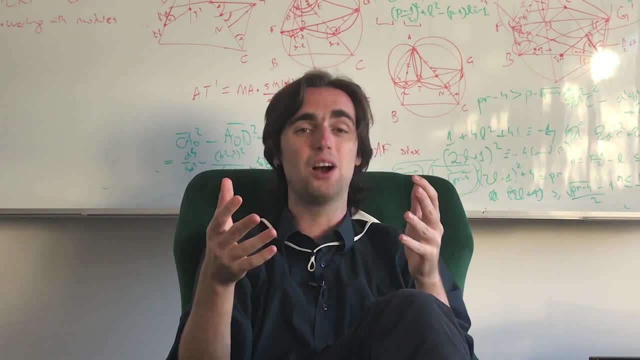 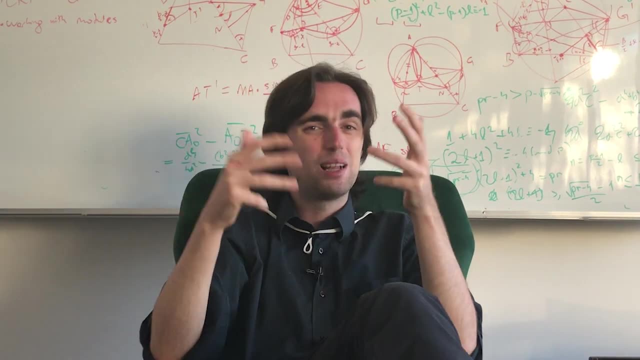 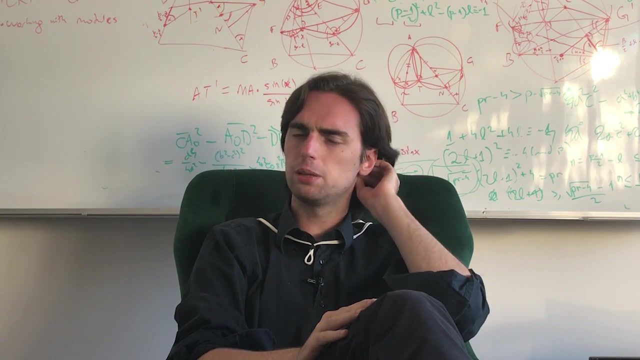 four different levels and there are beautiful problems in geometry that they can really teach you how you work with, like it can teach you new tricks that you can then apply to IMO level geometry problems. Other than that, there's also a Russian Geometry Olympiad- Scherrigan Geometry Olympiad. 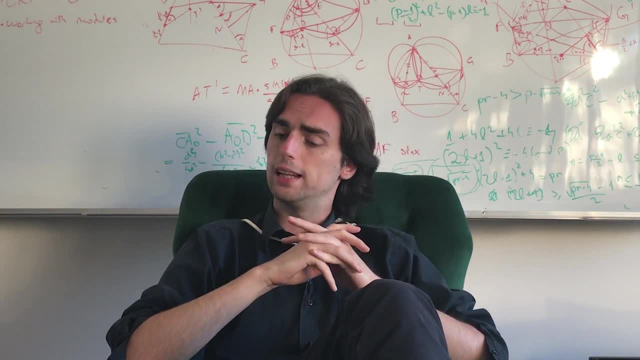 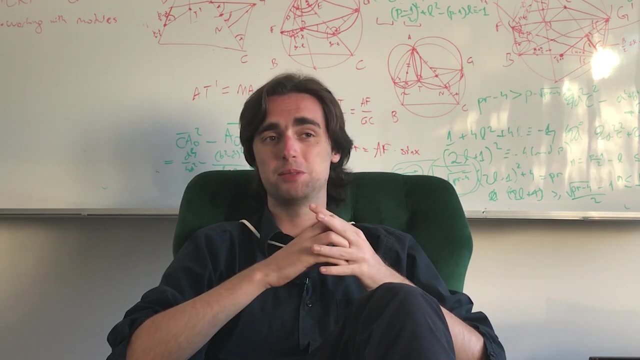 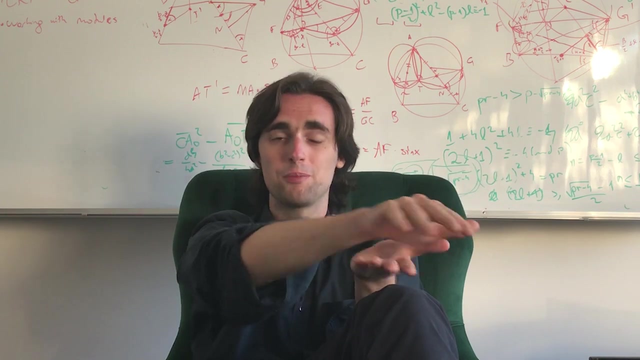 After that there's not much else that I know of that actually only has specifically geometry, but those two are absolutely great resources for good geometry problems, And there's always. you know, you need to look at problems from the level of competition that you're preparing for. 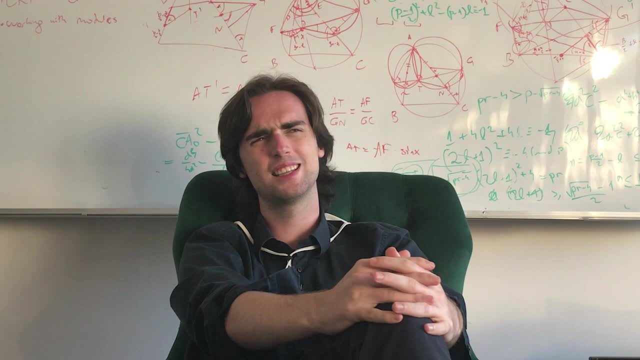 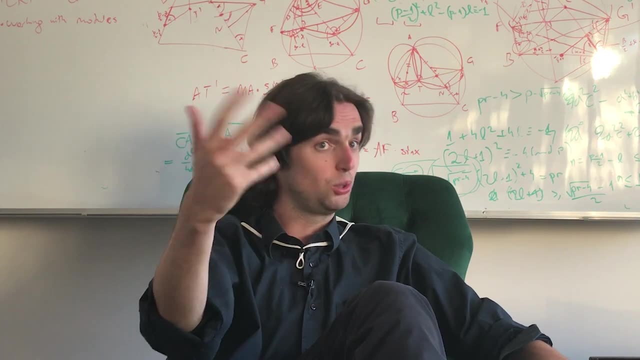 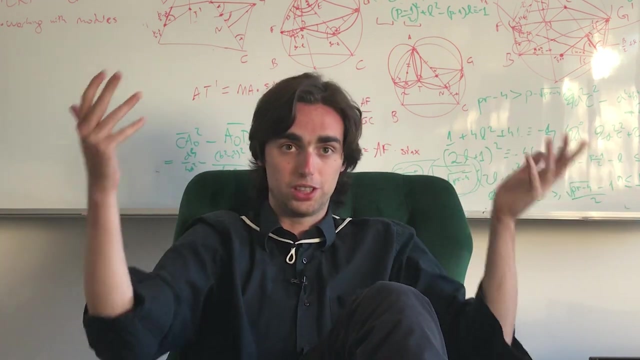 Given your country, given your level of competition that you're looking at, they might give you different types of problems. They might focus more on you demonstrating you have some knowledge, as opposed to you demonstrating you can solve problems. It's unfortunate because the IMO is usually you demonstrating that you know. 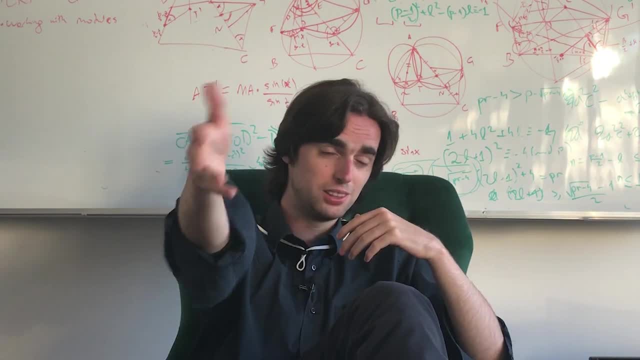 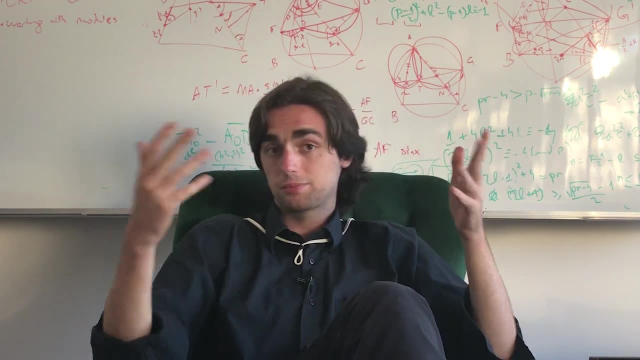 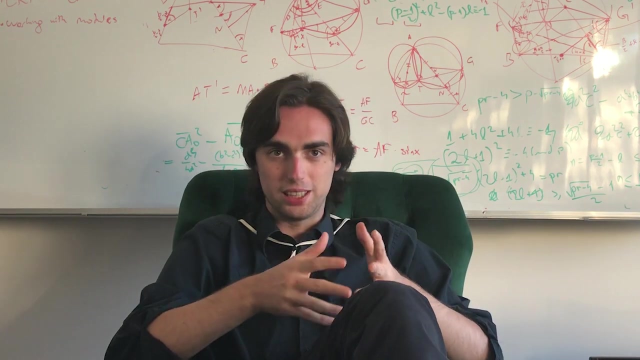 can solve some problems rather than that you demonstrate knowledge. But some competitions do need you to demonstrate a certain form of knowledge which you need to learn about And, again, this is best done through solving problems from that competition. That's really all you need for geometry in math competitions. 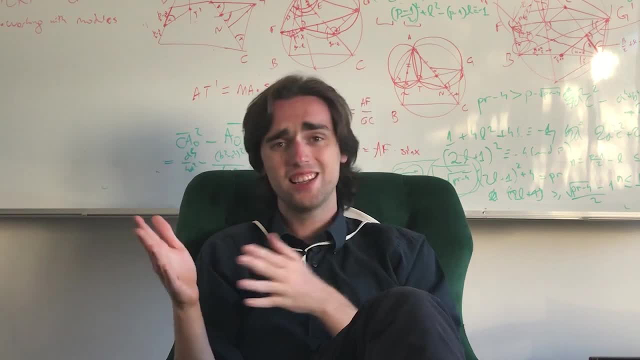 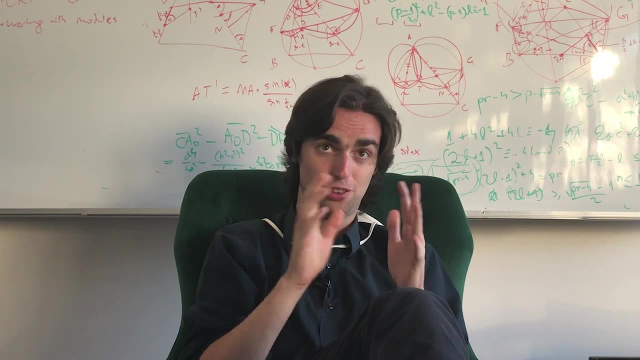 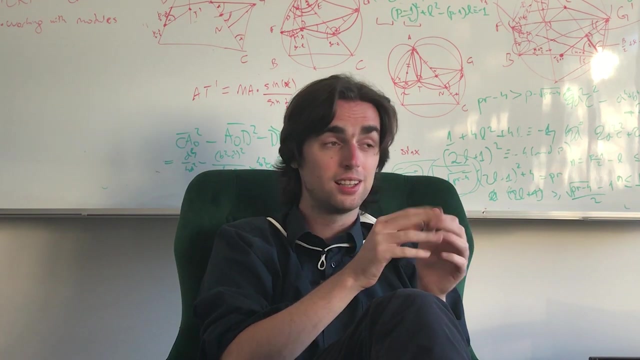 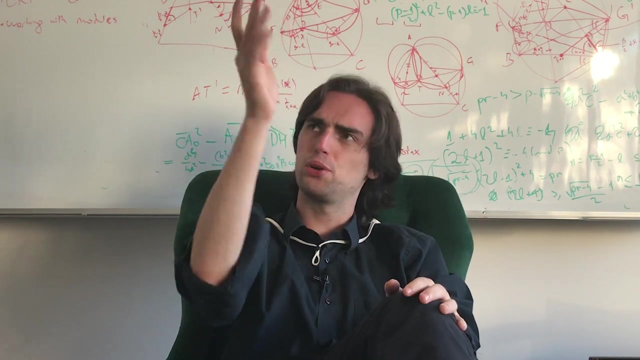 geometric lemmas, which is pure gold, And other than that, you need to solve problems, as with everything, And a good competition for geometry Olympiads- actually for geometry types of problems- are the Iranian Geometry Olympiad. This actually exists. It's a competition that only has geometry problems And you can try to solve problems from there in three or 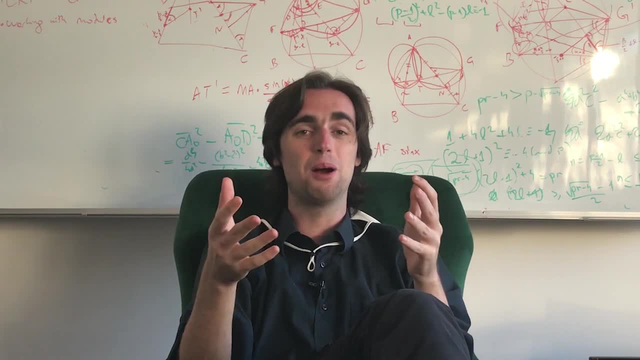 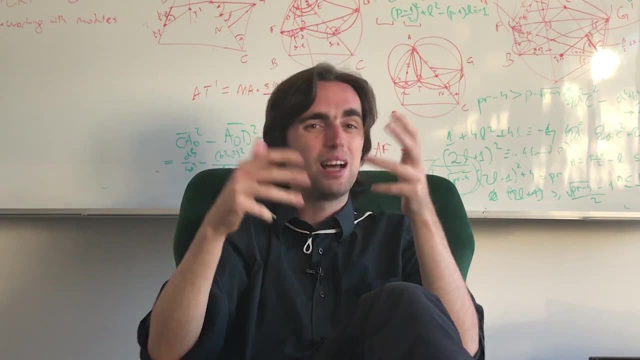 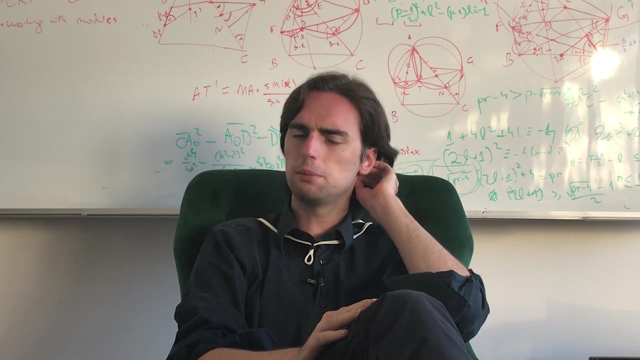 four different levels And they're beautiful problems in geometry that they can really teach you how you work with it, like it can teach you new tricks that you can then apply to IMO level geometry problems. Other than that, there is also a Russian geometry Olympiad, Sharigin Geometry Olympiad, And 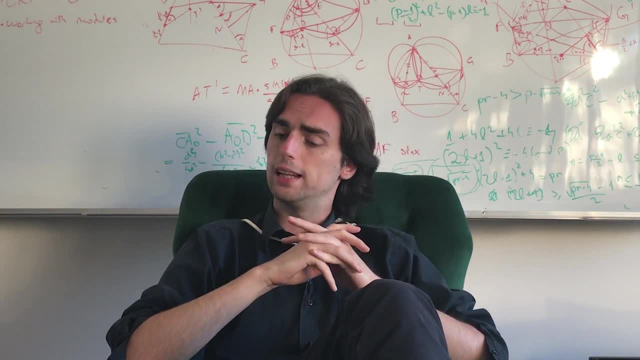 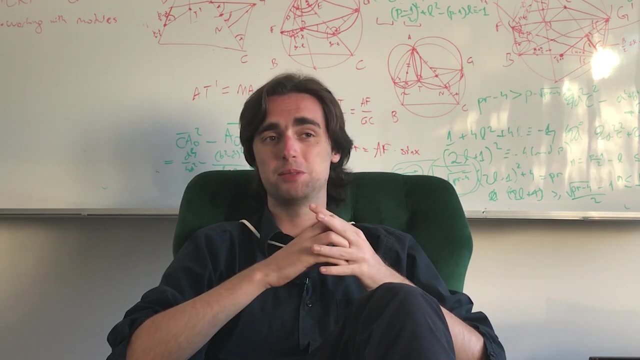 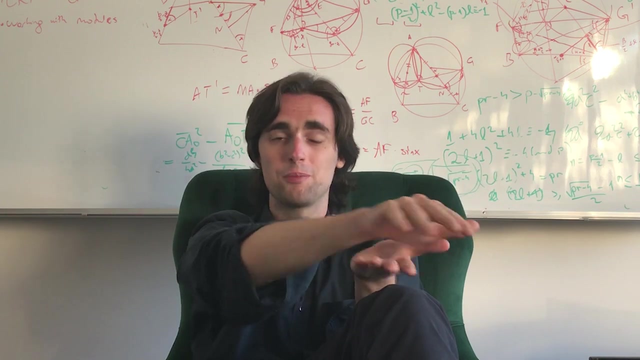 After that there's not much else that I know of that actually only has specifically geometry, but those two are absolutely great resources for good geometry problems, And there's always. you know, you need to look at problems from the level of competition that you're preparing for. 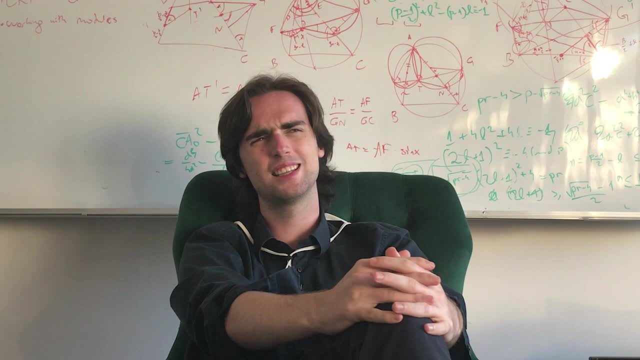 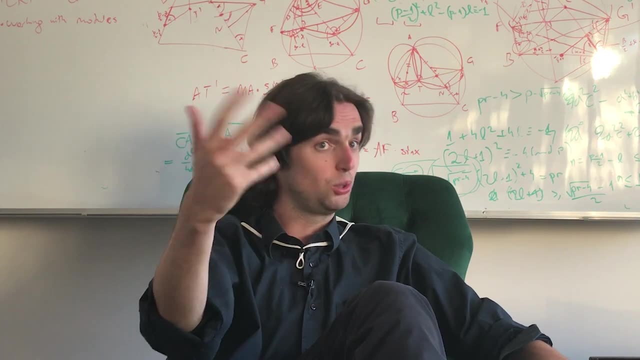 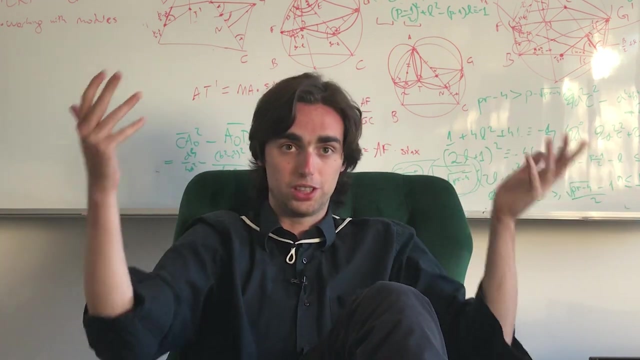 Given your country, given your level of competition that you're looking at, they might give you different types of problems. They might focus more on you demonstrating you have some knowledge, as opposed to you demonstrating you can solve problems. It's unfortunate because the IMO is usually you demonstrating that you know. 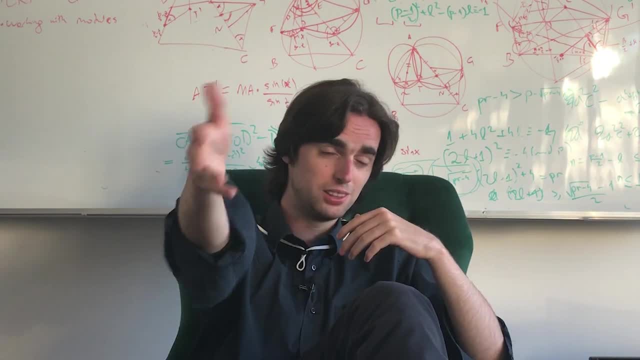 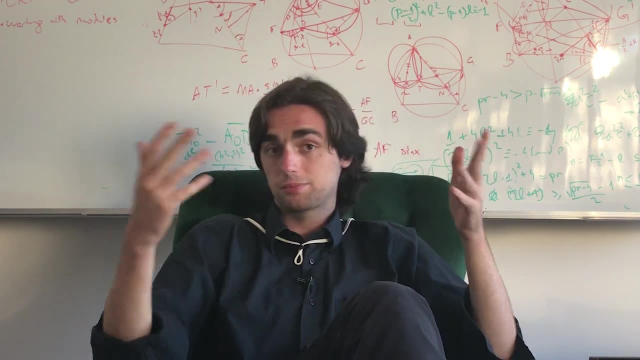 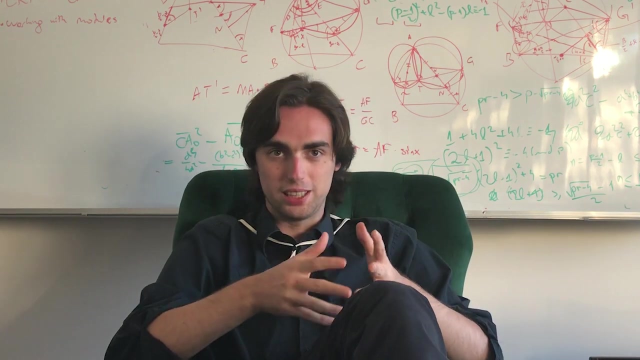 can solve some problems rather than that you demonstrate knowledge. But some competitions do need you to demonstrate a certain form of knowledge which you need to learn about And, again, this is best done through solving problems from that competition. That's really all you need for geometry in math competitions. 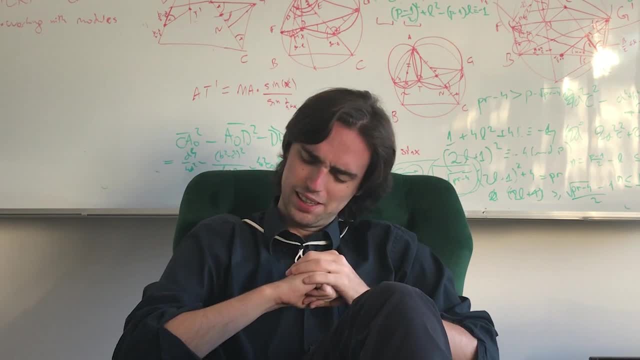 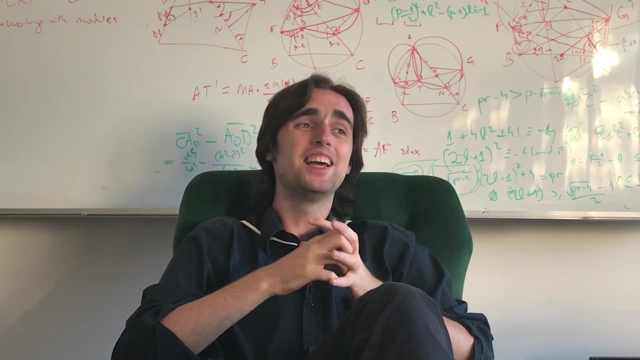 These are things That you can really practice, And I'll be honest here: When I started with math competitions, my worst area was geometry- The absolute worst. But at some point, at one point, I decided that wait, I'm not going to pass to the IMOs. 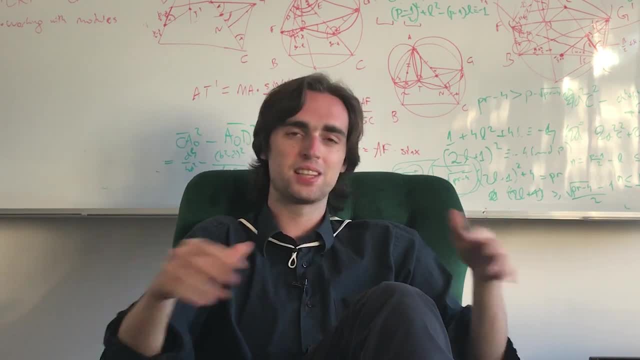 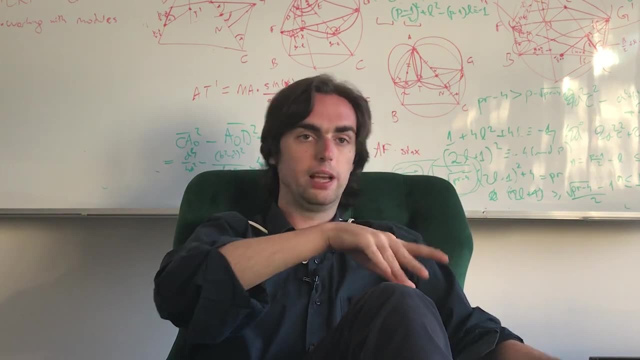 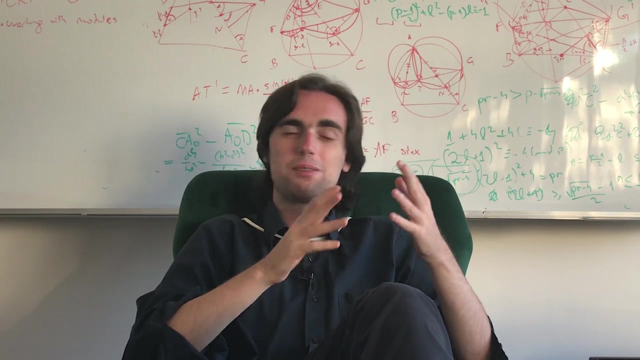 or it's going to be very difficult for me to do these competitions well if I don't learn enough about geometry. So I started learning about the basics- building blocks- slowly. I wrote a whole textbook for myself On why different things are true. what are the different lemmas? I know why are they true? 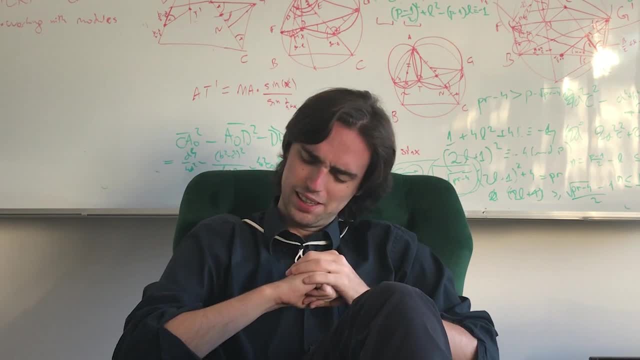 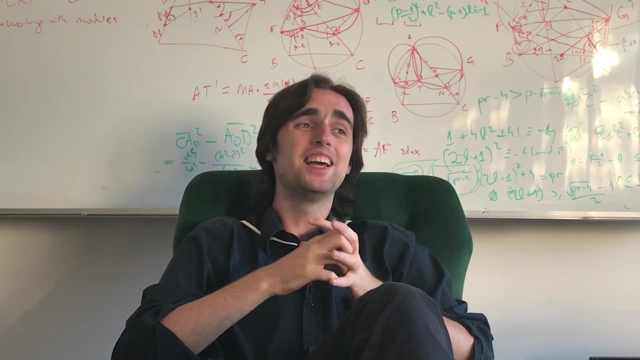 These are things That you can really practice, And I'll be honest here: When I started with math competitions, my worst area was geometry- The absolute worst. But at some point, at one point, I decided that wait, I'm not going to pass to the IMOs. 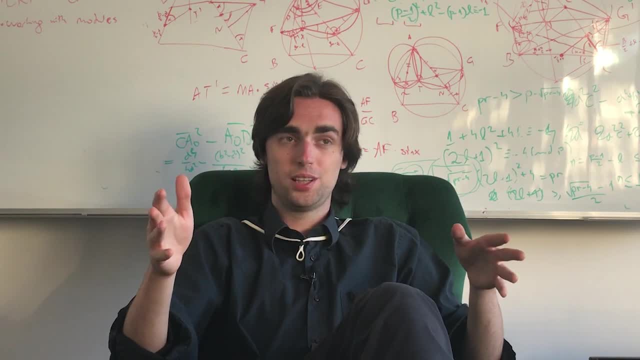 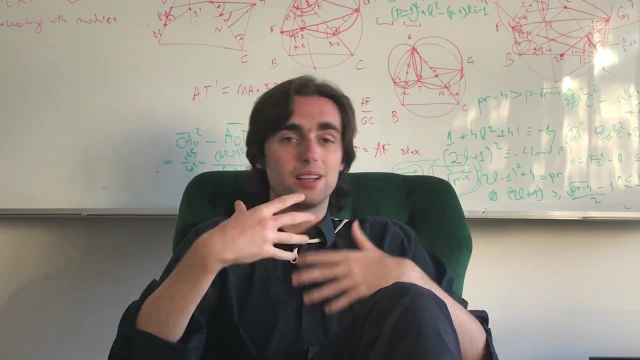 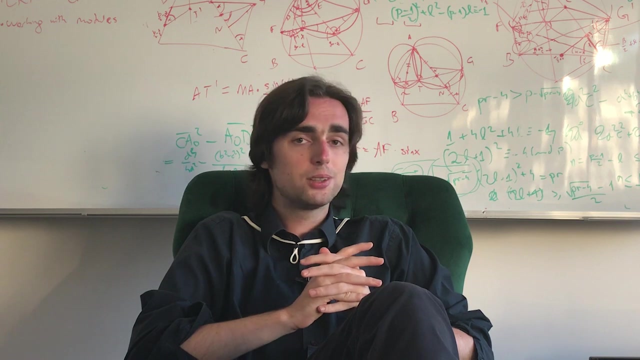 And I started actually solving problems that were a grade or two below me, that were not going to show up in my competitions but that I needed to solve to build up my confidence And at the end of the IMO, when I finished with my last IMO, I could solve the hardest geometry problem at the IMO.